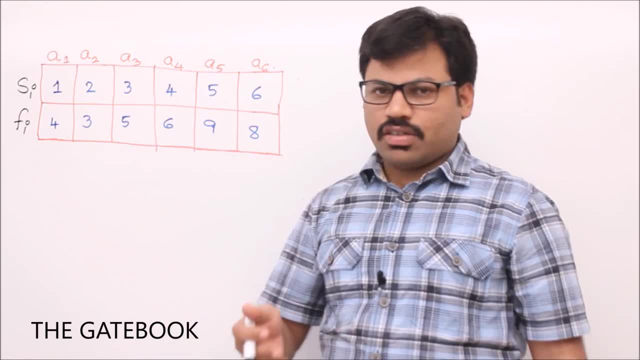 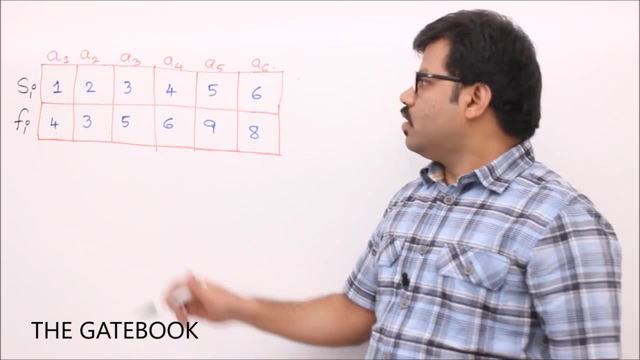 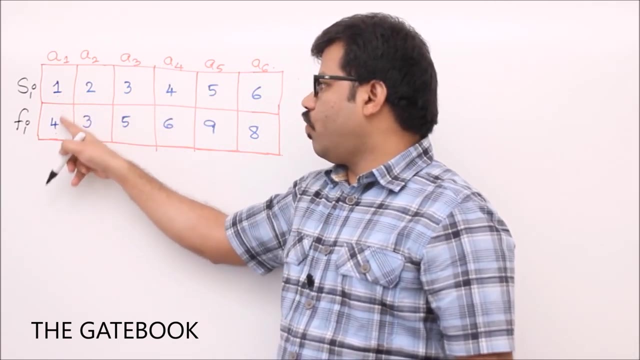 are given. that means so this may be an activity or, you know, a lecture maybe, so that lecture is happening at one o'clock and it is finishing at four o'clock. in that way, so we can imagine all these things as lectures, okay, some delivered by some faculties, so the duration is one to four. 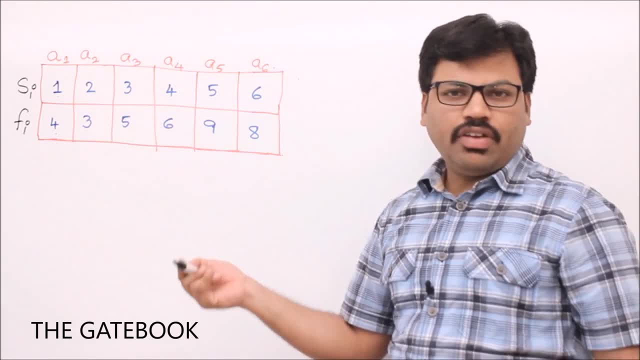 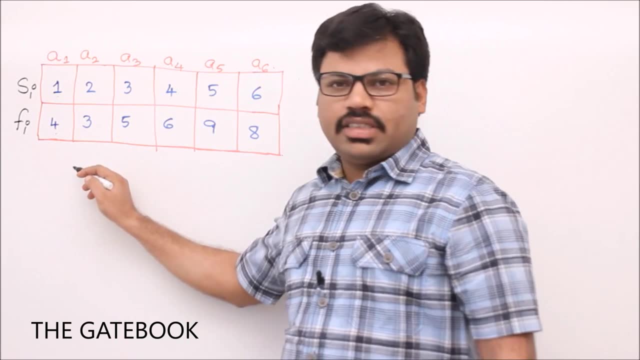 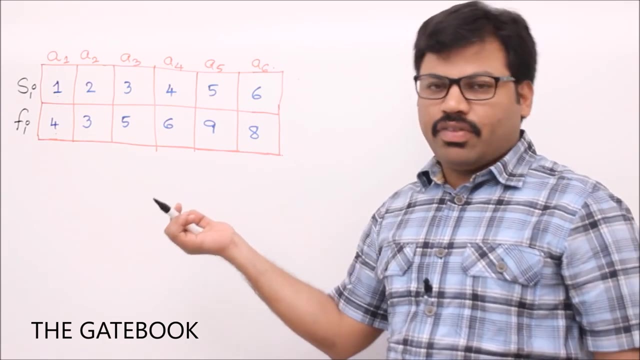 this duration is two to three. in that way every lectures duration is given for that starting time and finishing times are given. so now what we have to do here is our problem is here: optimization, like dynamic programming. already i told you there is no much difference between this dynamic programming problems and greedy method. every this problem also will have. 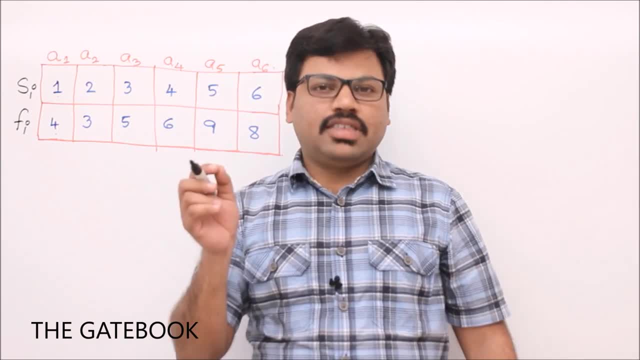 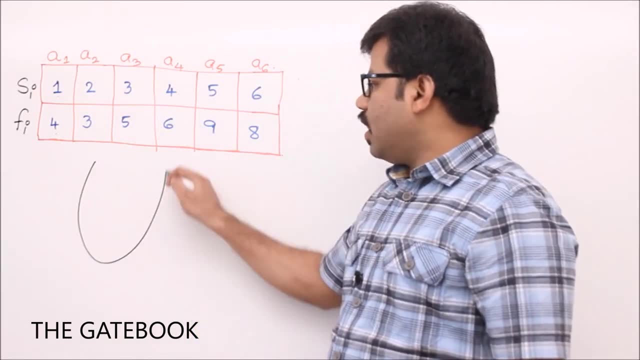 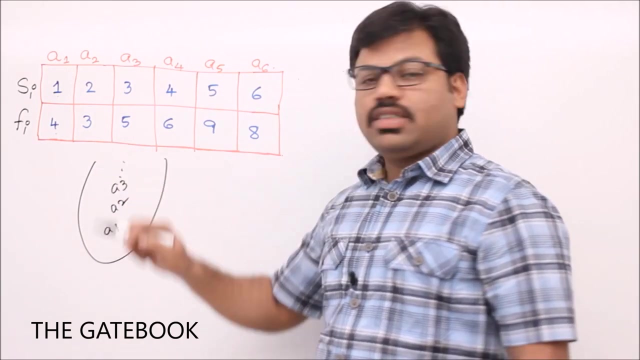 optimal substructure. and here also we try for optimization, like minimizing something or maximizing. so what is the problem here? i will tell you you will. you will be given a bag in that you have to collect the activities, something such a way that the number of activities should be maximized and these activities should satisfy one condition. 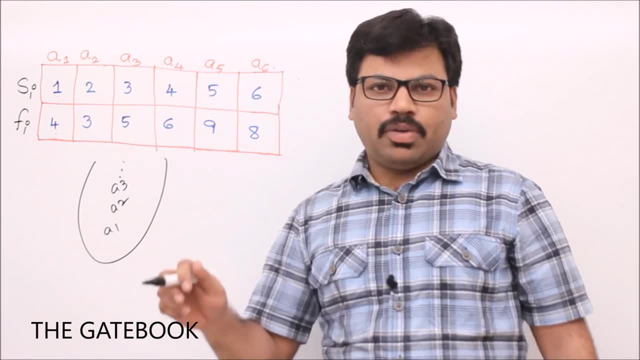 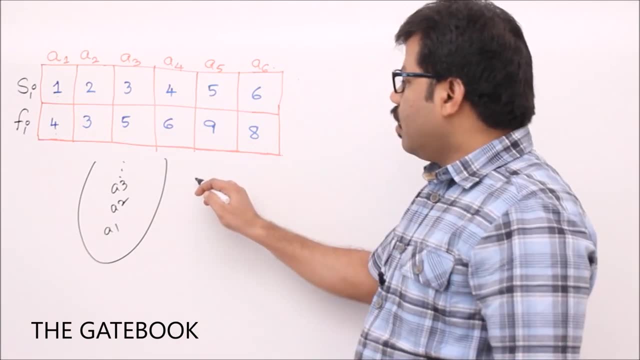 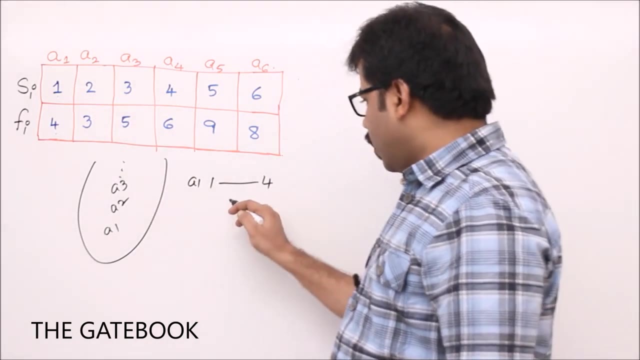 which is important, condition, that is, they should be compatible. two activities are said to be compatible if there there is no overlapping of timings. example: a1 is one to four, correct, let's draw like this: this is the timeline now. a2 is two to three: see here. so two to three, right then there. 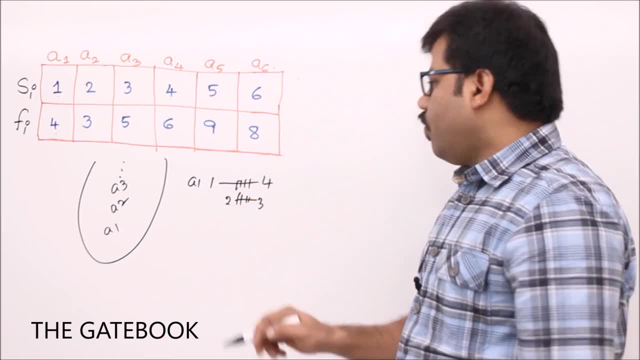 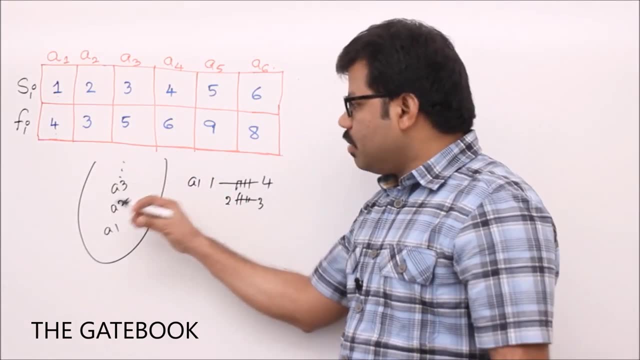 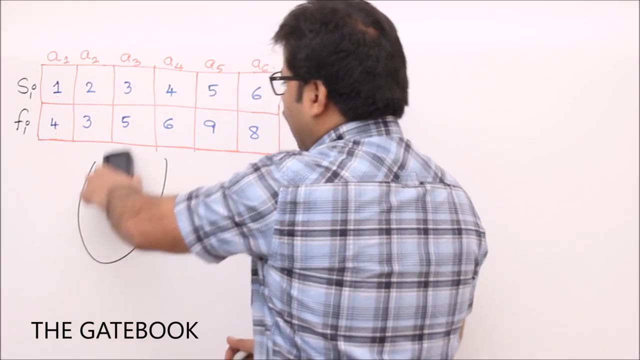 is a overlapping correct here. if any two activities doesn't have this kind of overlapping, we say they are compatible activities. now we have to find out you know maximum number of compatible activities possible for given these durations. we'll see the in this problem. what are the maximum number of activities we can have at a time? so let me start with a1. if 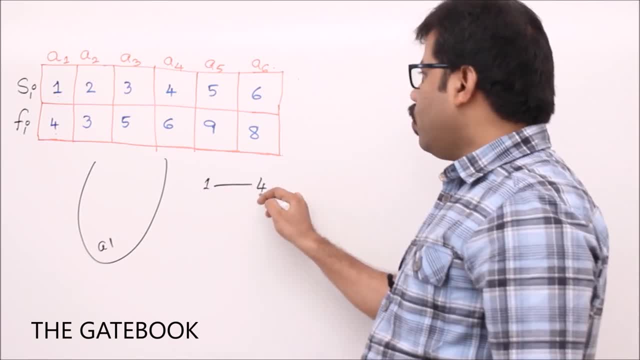 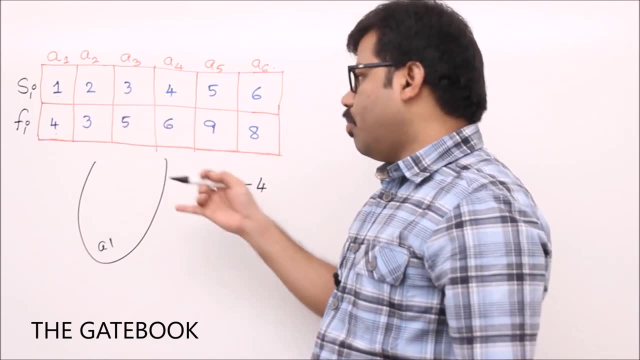 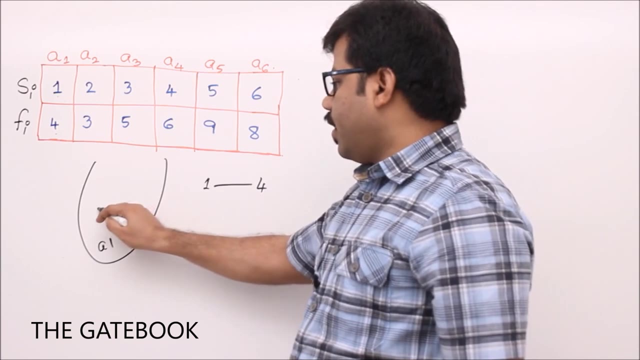 i take a1, which is one to four. let me show here one to four, then i can't take two to three thing right, then i can take. can i take a3? no, still it is three to five. compare not compatible. now we can go for a4, which is four to six. what if i take a5? let's try. if i take a5, then it is going to be from five. 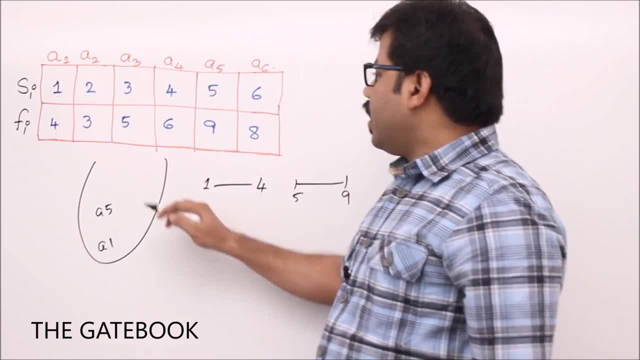 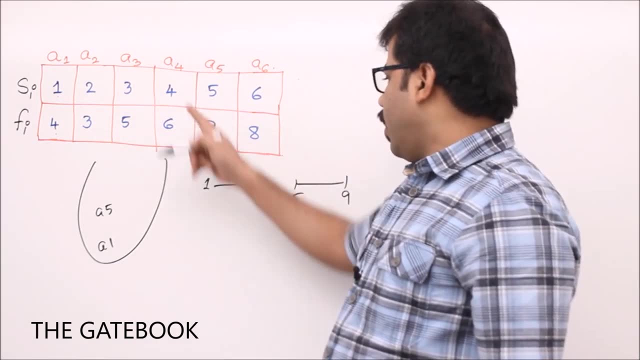 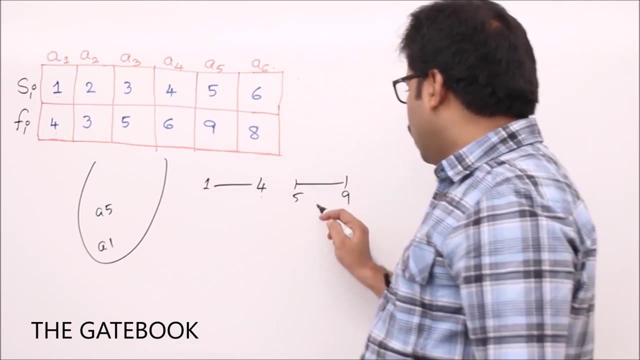 to nine, correct. now, after taking a5, can you take anything? so can i take a2 already? i cannot take a2 correct now. a4 already we have not taken, but it is four to six. it overlaps with this a5. so six to eight, this will again overlap with a5. that's why these two are compatible activities. but is it? 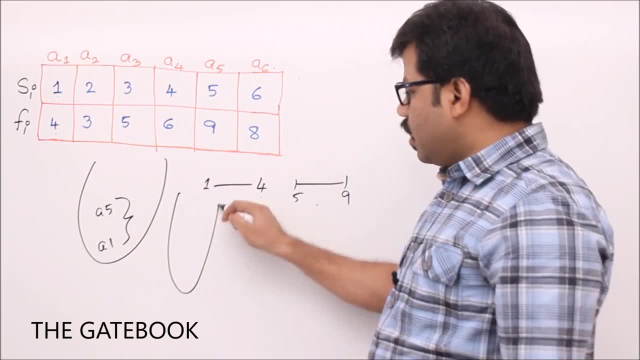 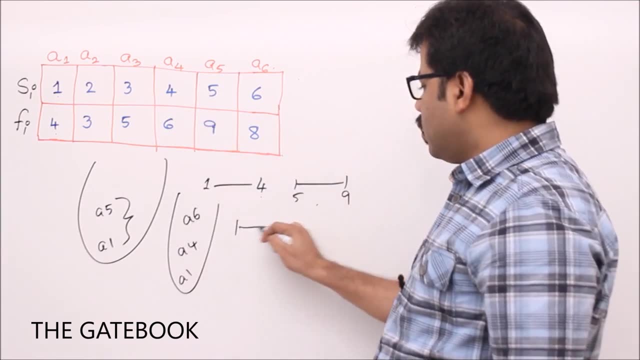 maximum, or we have any better choice. yes, we have a better choice. that is, take a1, one to four, then a4, four to six, a6, six to eight. so this is the picture: one to four, then four to six, then six to eight. so the activities are a1, a4. 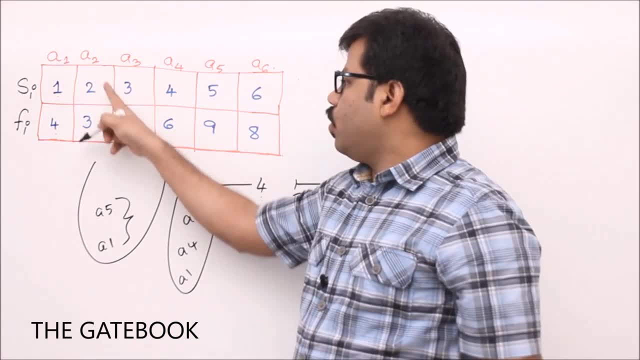 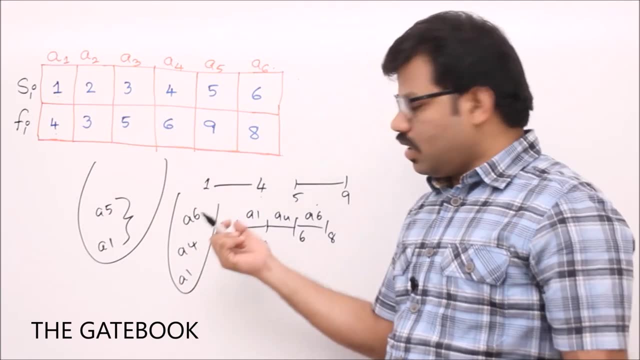 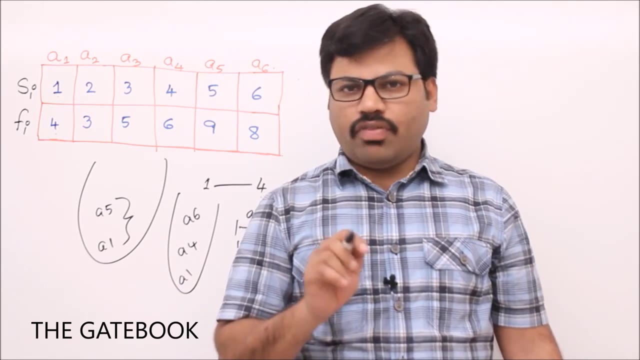 a6. similarly, we have another option also: we can take two, three, three, five, five, nine. otherwise, two, three, three, five, six, eight, so a2, a3, a6 or other thing, right. so we have lot of possibilities. but our question is: we have to find out one set of such maximum number of activities. i don't want. 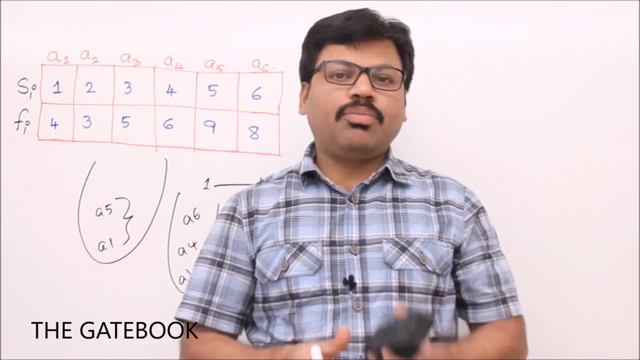 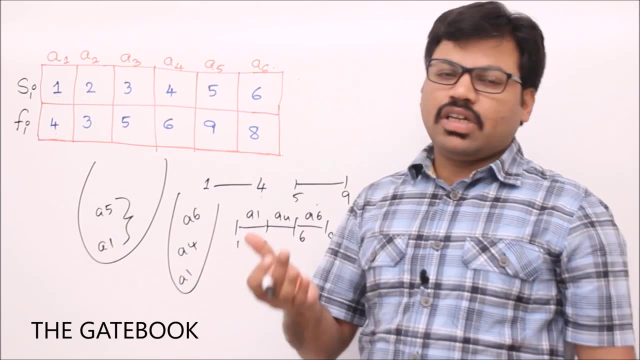 to compute all possible. i mean sets. i want to compute only one set, but that should be maximum set. so here we are, maximizing the number of activities which are non-overlapping, otherwise compatible. we'll see how to solve this problem. what we are going to do is we are going to 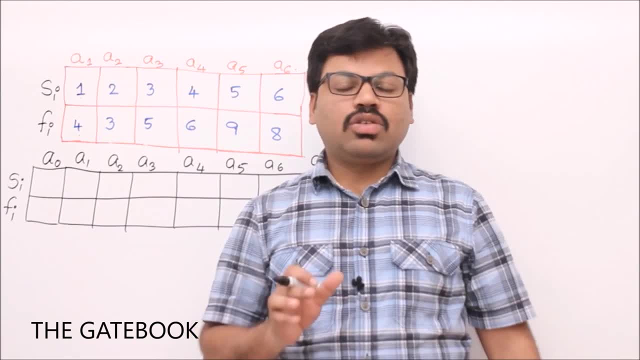 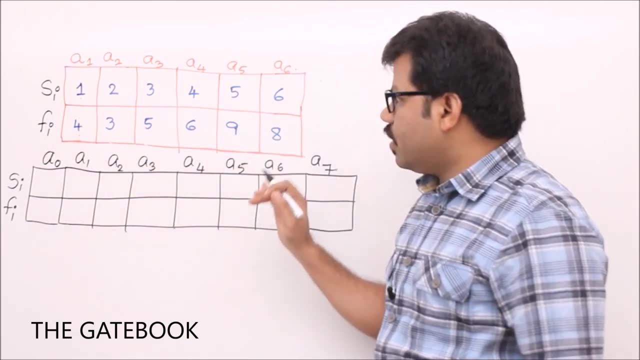 order the activities based on their finishing times, so that you know problem will be easy for us. let me do that first. so here, activities. if you see, four, three, five, six, nine, eight are finishing times, right. so what is the first activity? who has finishing time earliest, which is a2, correct, let's? 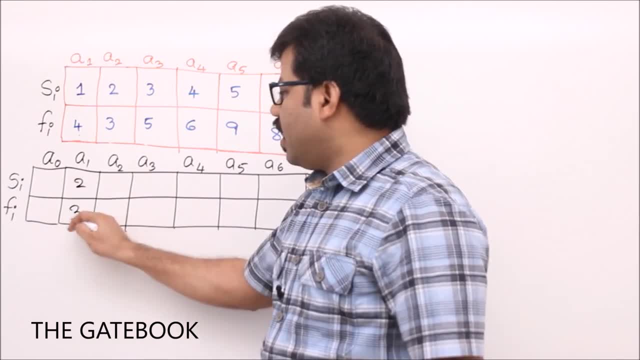 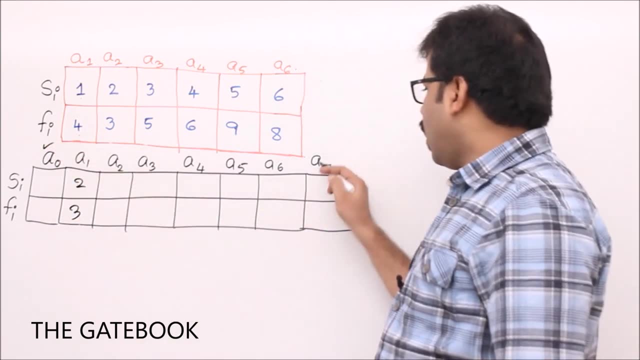 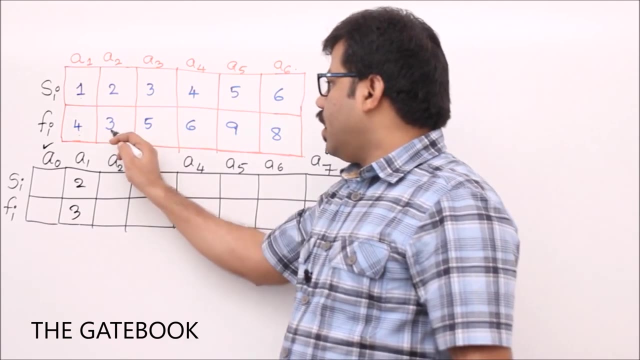 write here. what is that? two comma three. okay, i'm renaming the activities, so a1 is nothing but an activity whose finishing time is a2. earliest i'm ignoring- a naught, i will tell you the reason. and this last place also i'm ignoring, so you'll understand that later. so i let me use only these positions. next three, after that four. 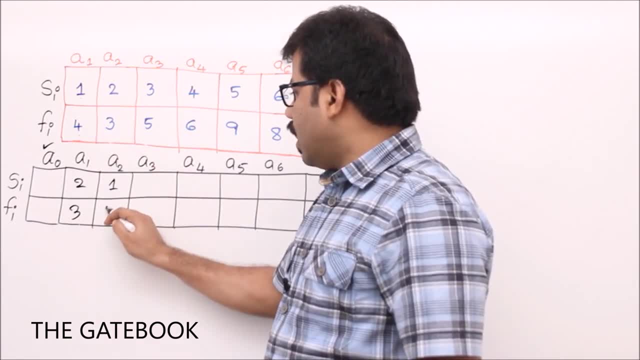 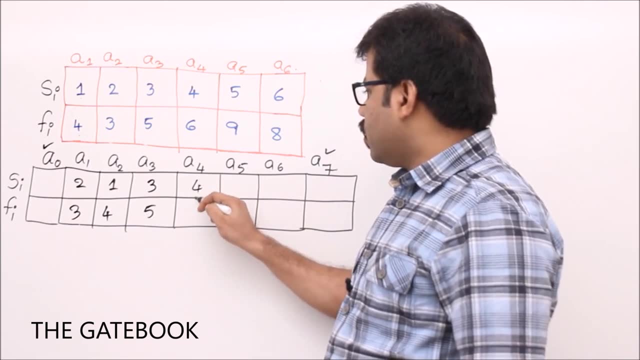 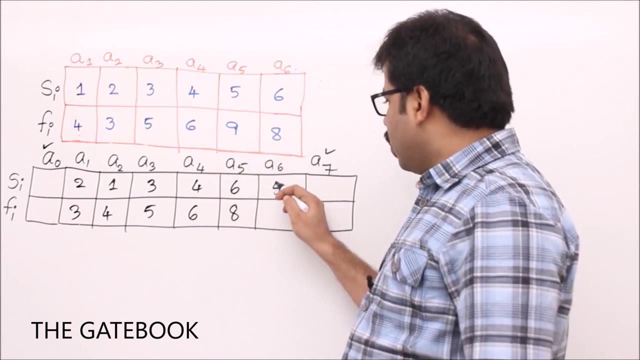 right. so four means what? a1, which is one to four. after that let's take three to five. then next finishing time is six. a four, four to six, then six to eight. correct: a six then five to nine. okay, so don't worry about the order of starting time. 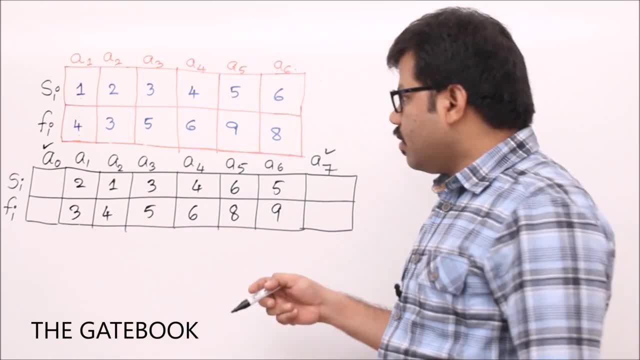 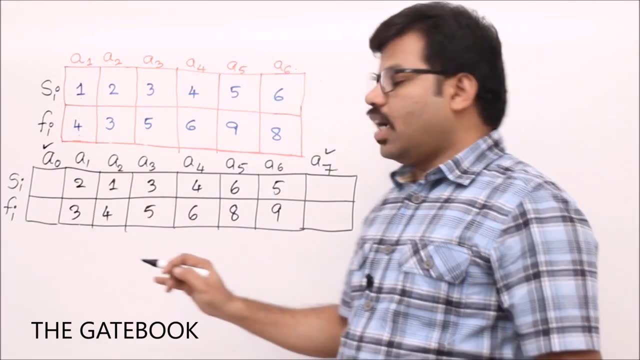 starting times: only see the finishing times once it is done. what we are going to do is we are going to add one activity- dummy activity here and dummy activity here, so that dummy activity is nothing, but it is going to start at zero and ends at zero. second activity: 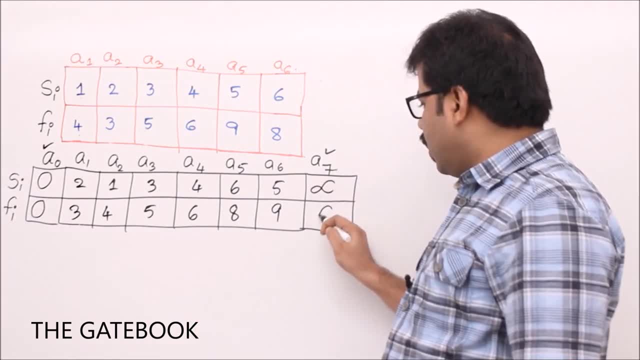 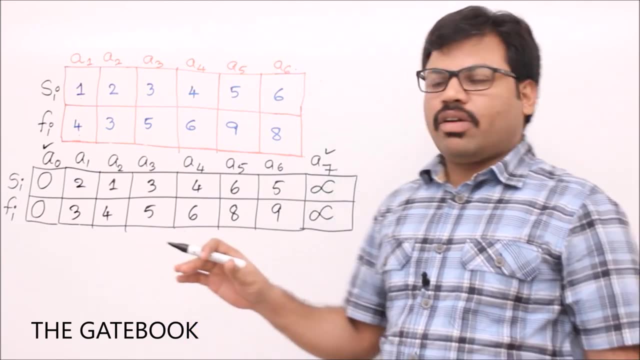 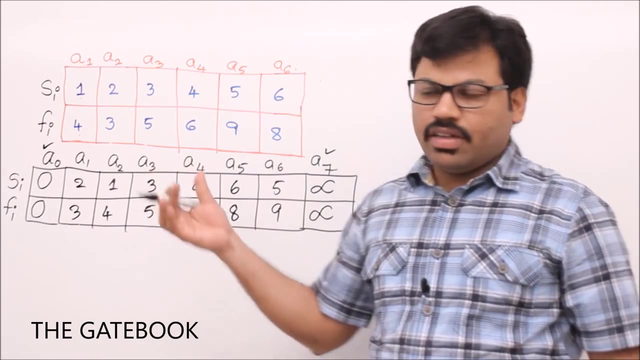 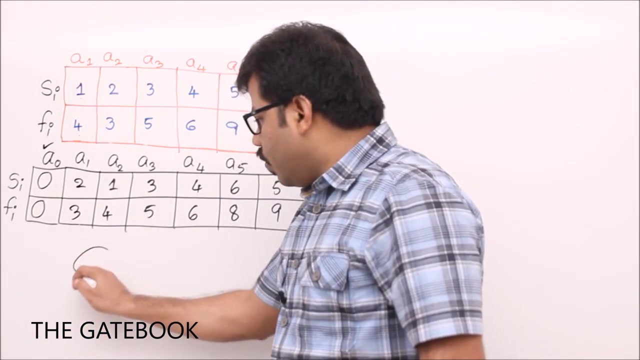 is going to start at infinite and finish at infinite, so in that way. so that's why that these two activities will not disturb our total problem. now we know that our total problem is maximum number of activities, otherwise the total number of activities which are compatible, correct for that. once you order the activities, you see this thing. i'm using a notation called. 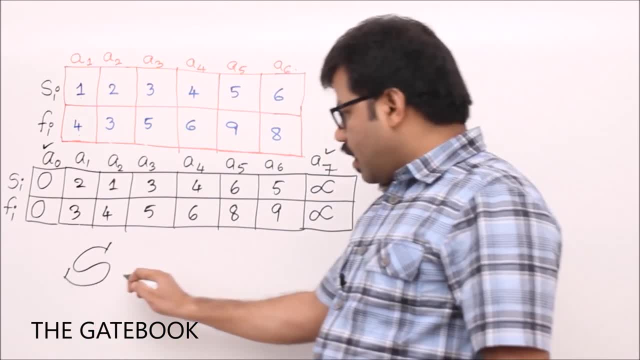 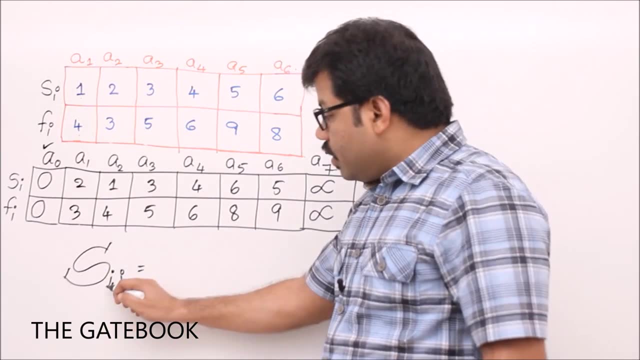 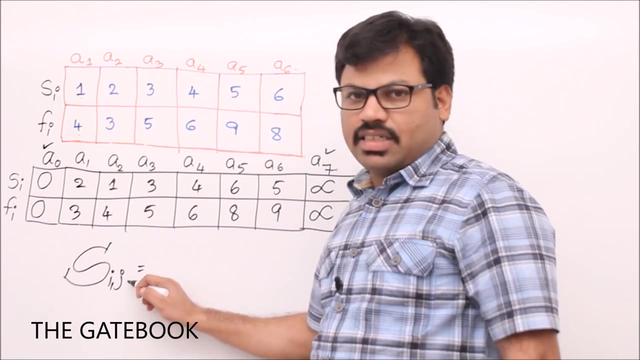 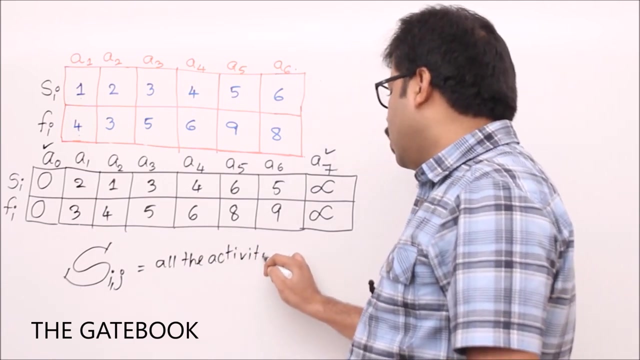 s from now onwards, try to understand it carefully. that is si j. what is sij is nothing, but it is a set, set of activities which starts after this activity i finishes and which finishes before the activity j starts. see, so I write it: all the activities. so it's a set, basically all. 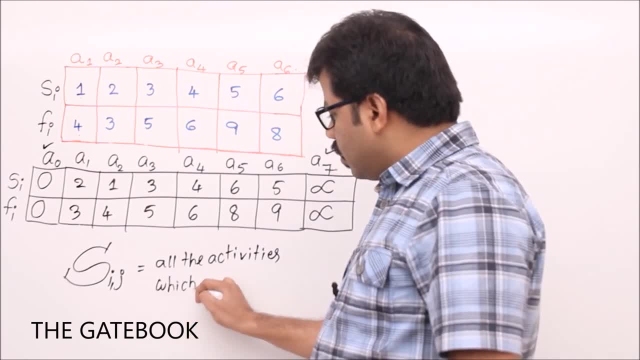 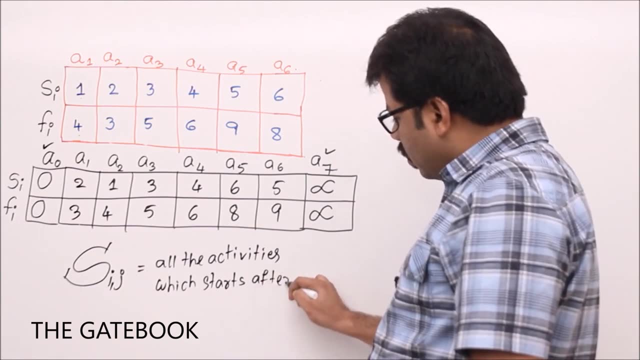 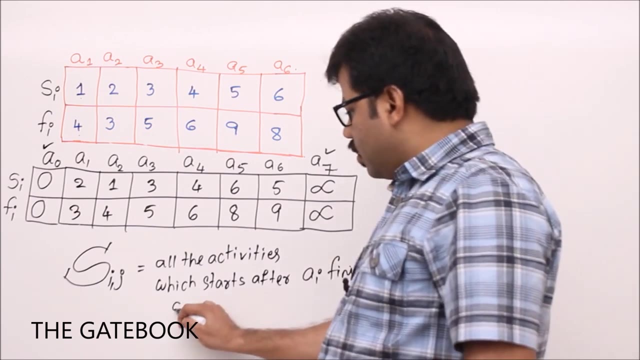 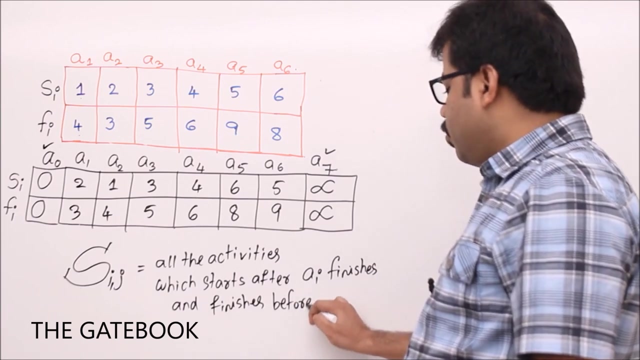 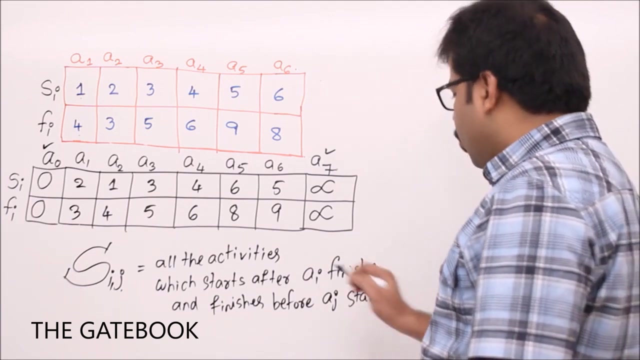 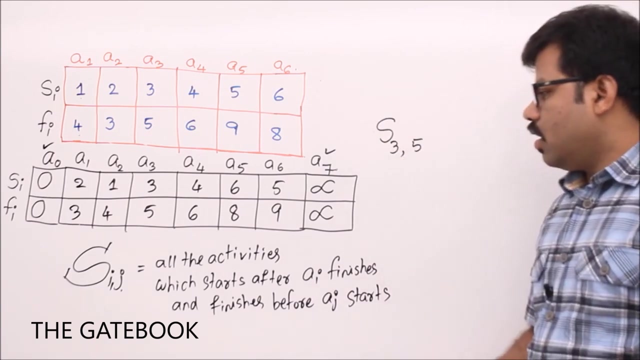 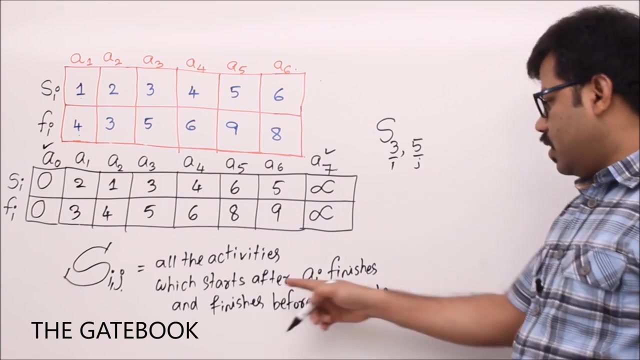 the activities which starts after activity a, I finishes and finishes before, finishes before this J means AJ, AJ activity starts. example. I will tell you what is s 3 comma 5. what is s 3 comma 5 is all the activities which starts after this. is I correct? this is J. let's substitute all the activities which 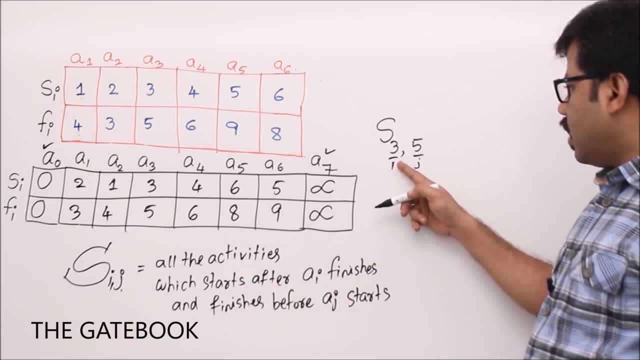 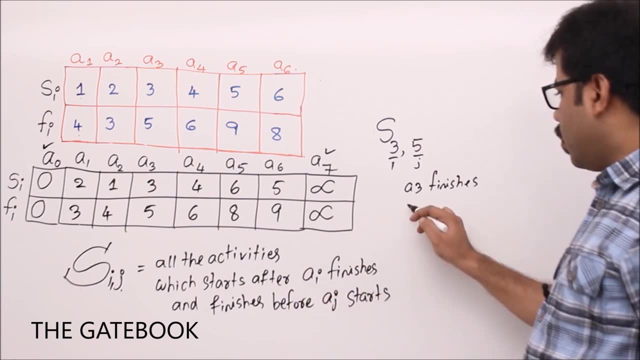 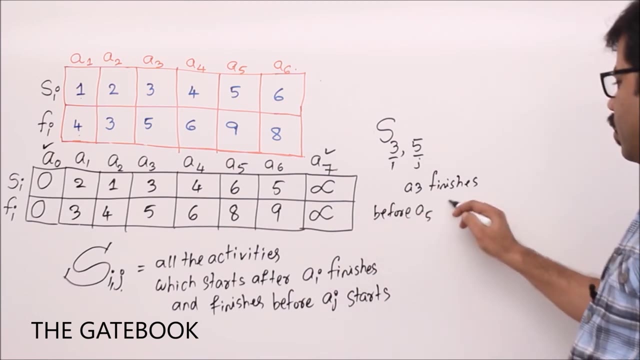 starts after AI finishes. here AI is nothing but a 3 after a 3 finishes, okay, and before AJ starts before AJ. so before here J is 5, a 5 starts. so please tell me what are all the activities we have which starts after a 3 finishes and after a 5 starts after a 3 finishes, when? 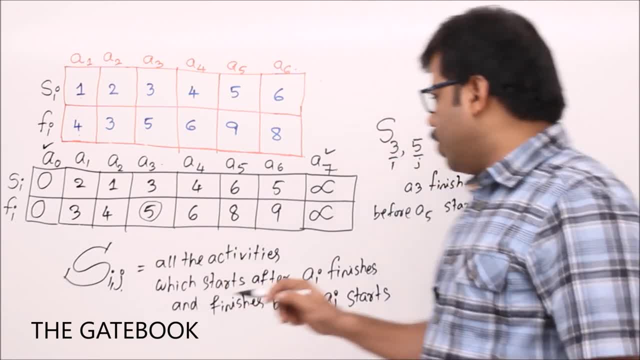 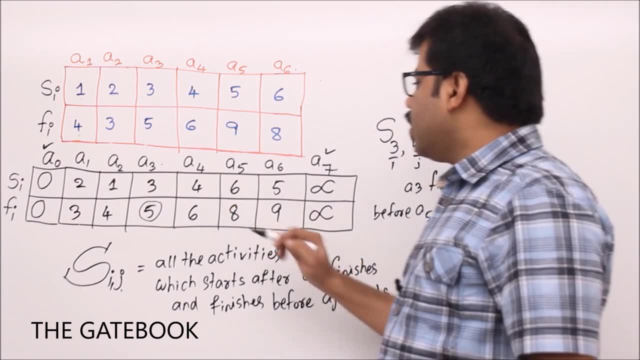 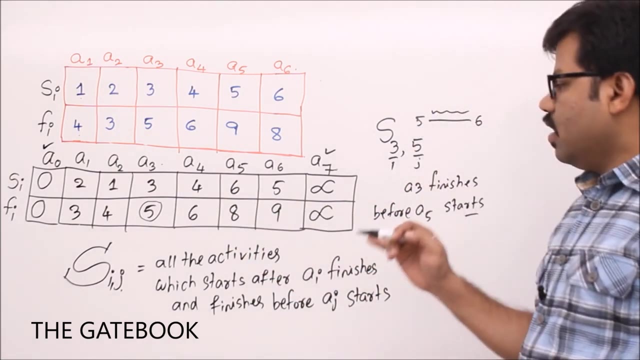 a 3 will finish. what is the finishing time? 5, correct? remember that means the timeline is 5: 2 before a 5 starts, when a 5 starts at 6 current. so before, that means now, in this interval, 5 to 6, there is no such activity. I think, right, yes, now let's. 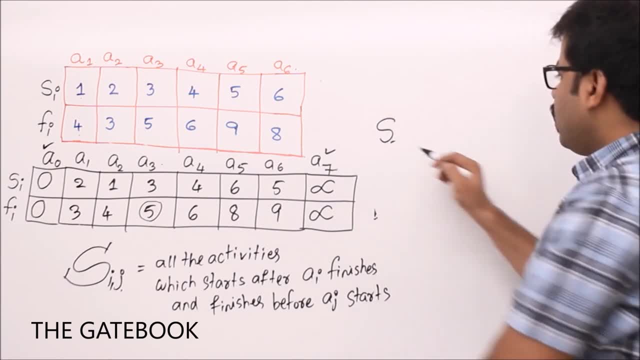 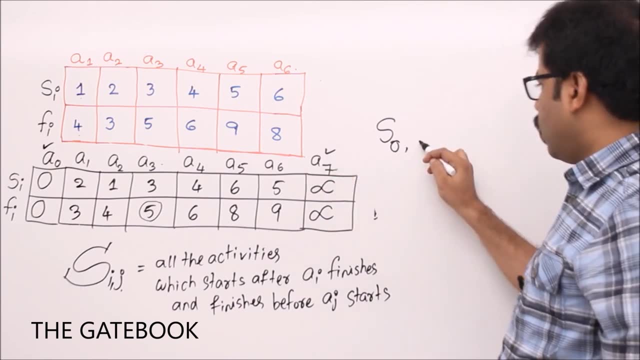 extend this s 3, 5, 2 little bit bigger. so what is s? let's say 0 to something, 7, we will see it's a very big thing, right? let's take 0 to 5 s, 0, 5, it is nothing. 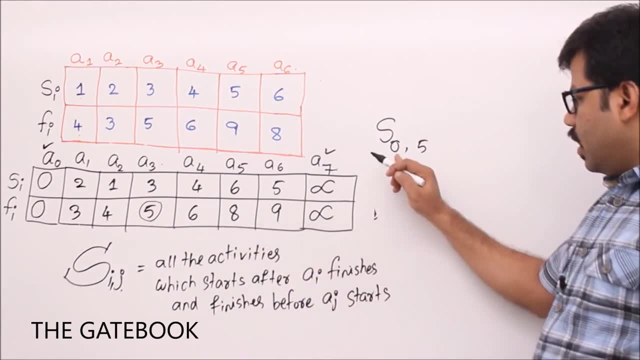 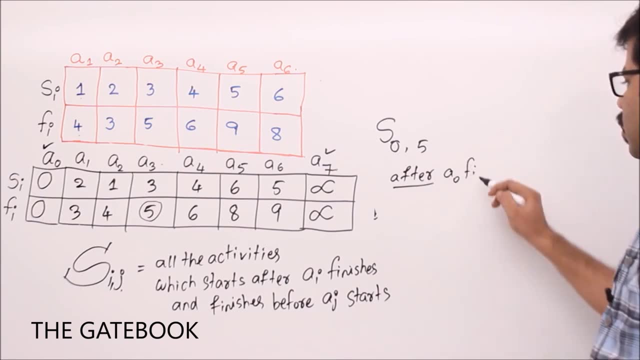 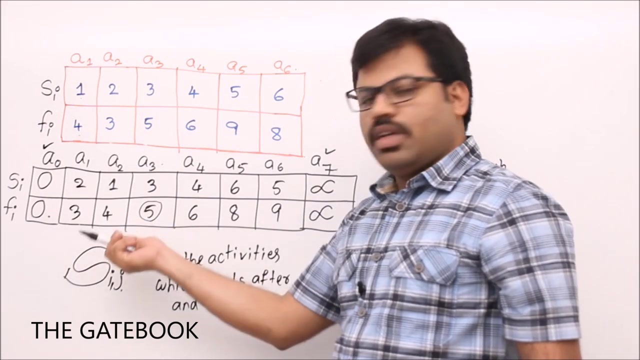 but all the activities which starts after a 0 finishes. let me like the crux, important thing: after A zero finishes, finish, and before AJ starts, here J is 5, 8, 5 starts. let's see, after A zero finishes, when will a zero finished? immediately write 0 to 0. that means so all the 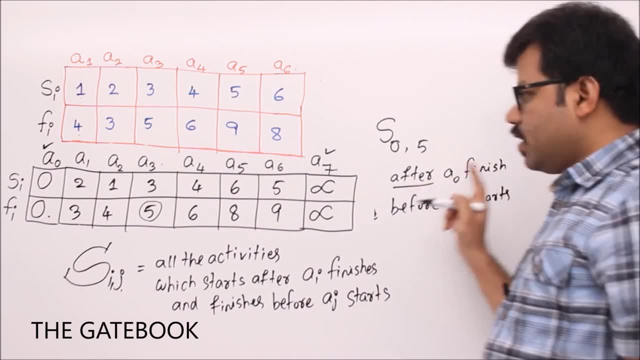 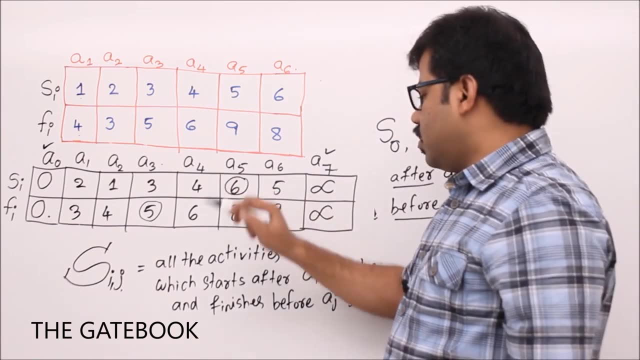 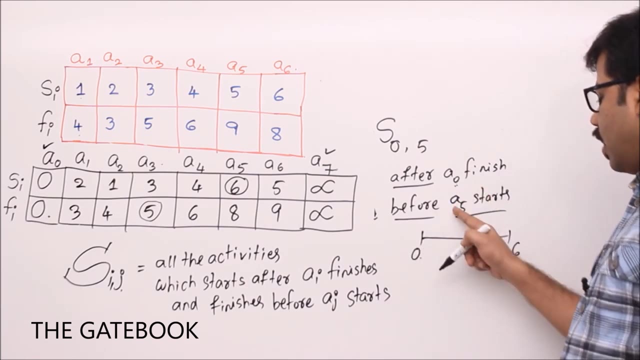 activities. so all the activities starts after AC approaches. I am tell me all the the activities before a5 starts when. when is a5 starting? 6, that means the time interval is 0 to 6. correct. finishing time of this a0 is 0. starting time of a5 is 6. in between, what are 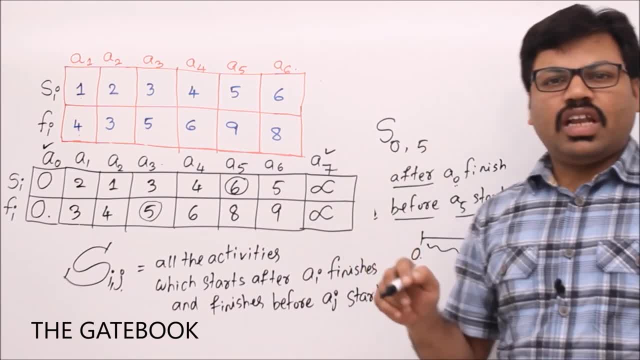 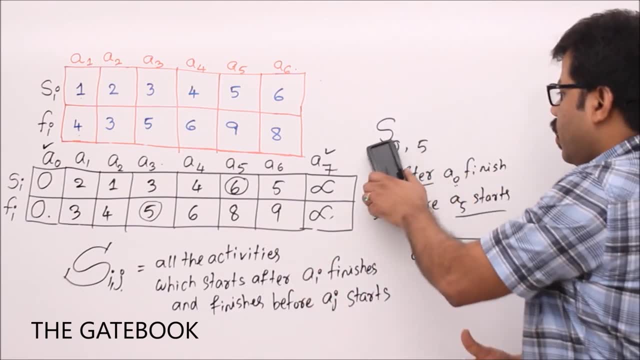 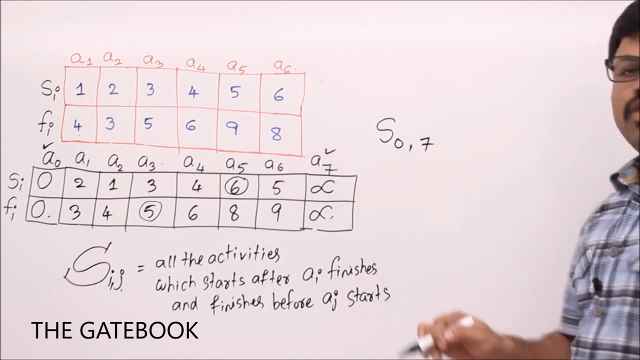 the activities you have. that is s05, you tell me. now i want to have all the activities into the picture. i want to consider all the activities. then what is the notation? very simple, right starting point 0, index comma 7. so what is s07? we'll try to understand all the activities. 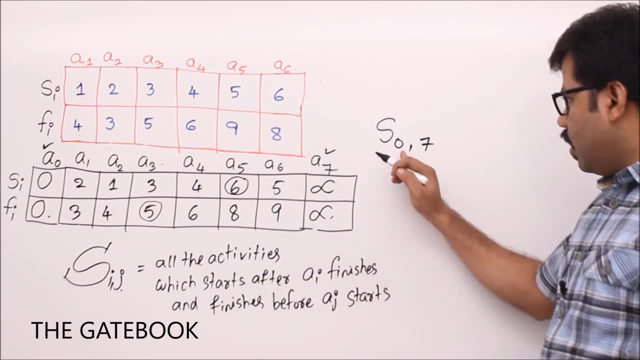 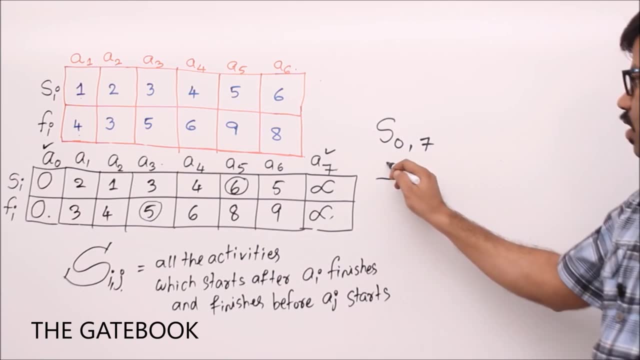 which starts after a0. here 0 i mean 0, right a0 finishes. a0 finishes means at 0, it finishes. this is the activity. a0. it starts at 0, ends at 0, correct, then? after 0. a0 finishes means 0 is the. 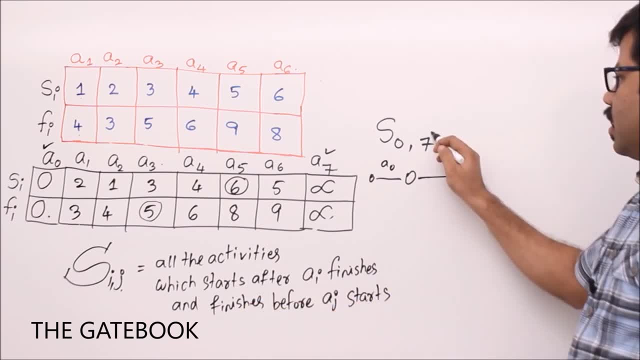 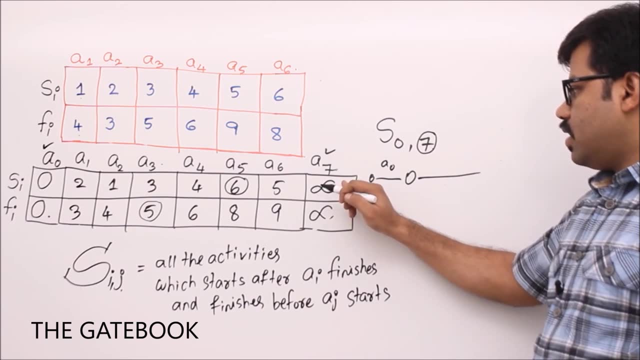 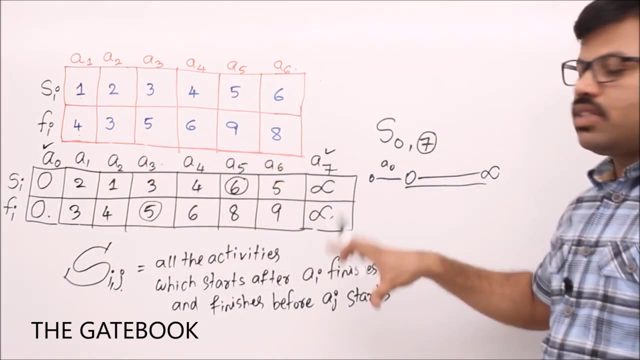 time and finishes before a j starts, finishes before a s0. this aj starts here. 7 is the j, a7 starts. when is a7 starting? infinite: that means between 0 to infinite. tell me all the activities. yes, it covers everything. that is why we are using a0 and a7. 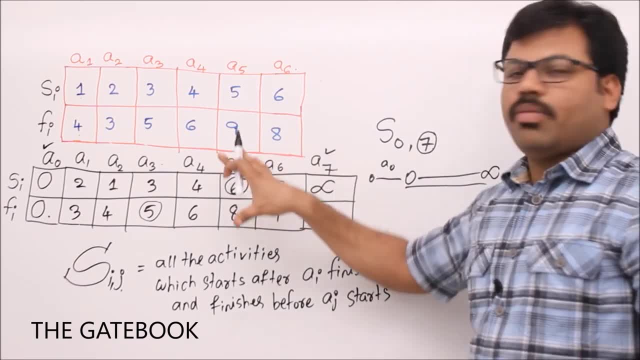 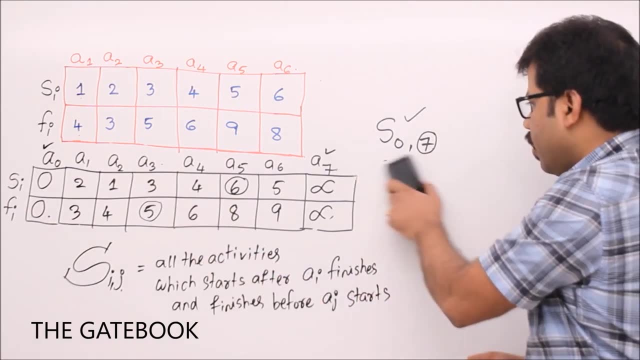 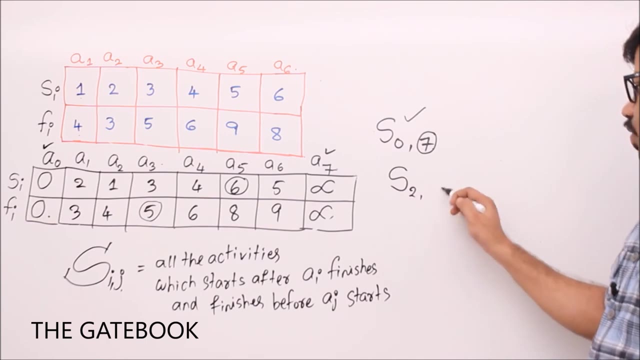 to represent our set or to our problem as a set. we are representing s07 to represent total set. understand. so we got come, i mean we got the comfortability with this s07 or any sij- correct one more time. we will try. what is s2 comma 6? we will see all the activities better. i write the. 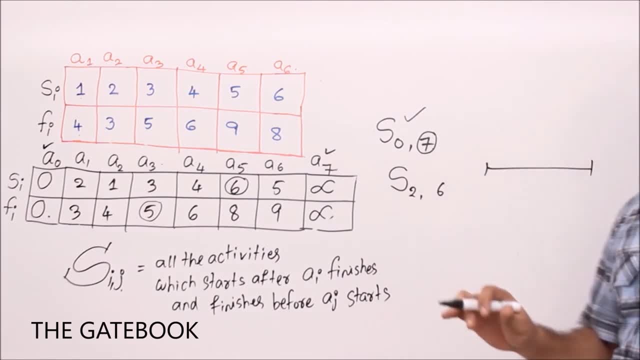 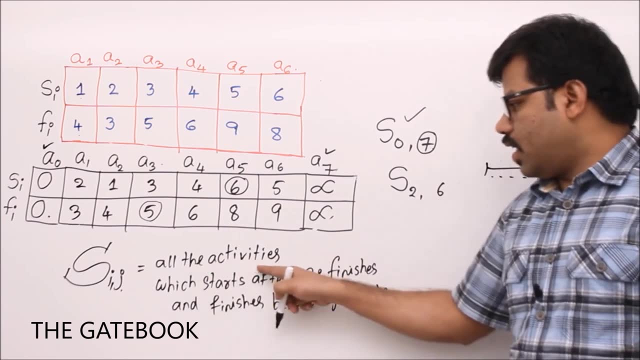 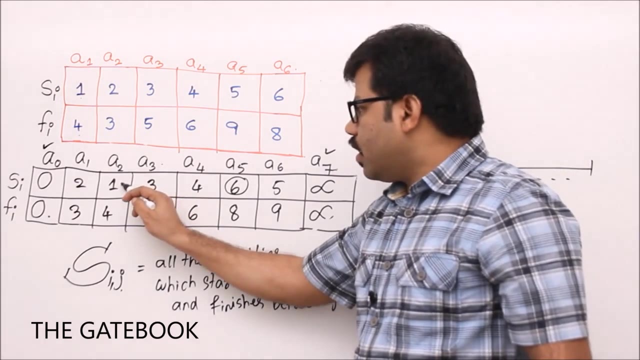 interval, time interval. so it is a time interval. all the activities are in this. in between this time interval, what is s26? all the activities which starts after ai, finishes ai is what here? a2 after a2 finishes. when is a2 finish 4, right? so that means we should start after 4 and before. 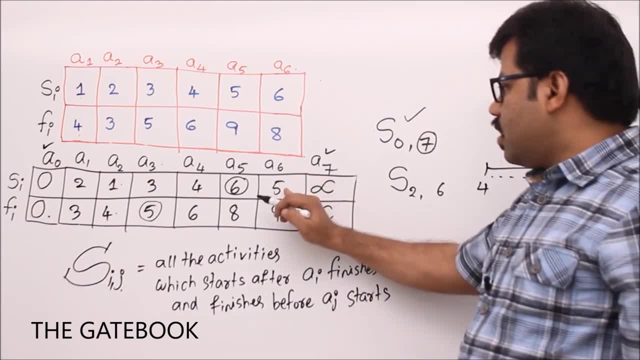 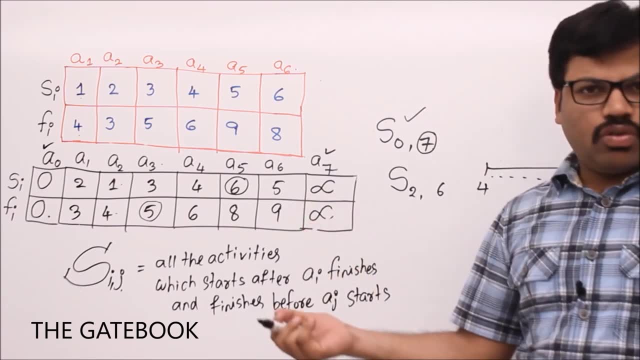 aj7 starts here before a6 starts. a6 starts at 5, then again 4 to 5 interval. in this 4 to 5 interval do we have any activity? of course no, but it is empty set right. so this is about s2 6. so i am explaining. 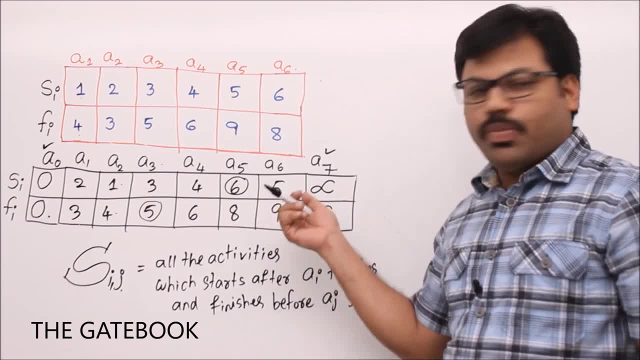 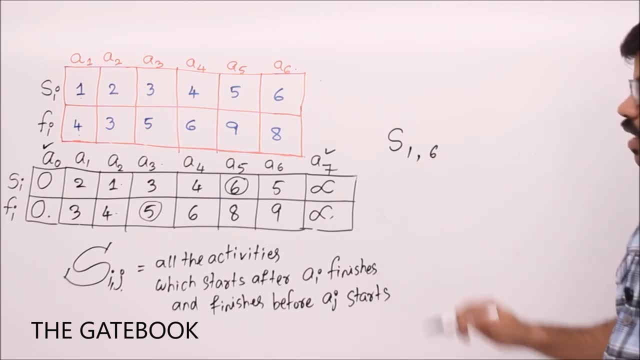 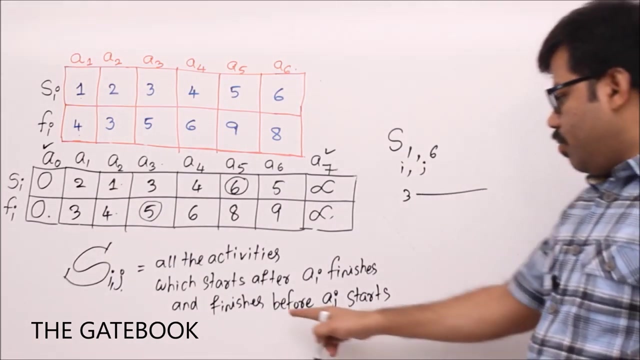 you these things. the only reason is: this is very important. now we will see one more time. s1 comma 6 ready. so what is s1? 6 is all the activities which starts after this. this is i, this is j. after a1 finishes here, a1 is uh. this one right a1 finishes 3, 3, 2. and before aj starts, aj is a6. 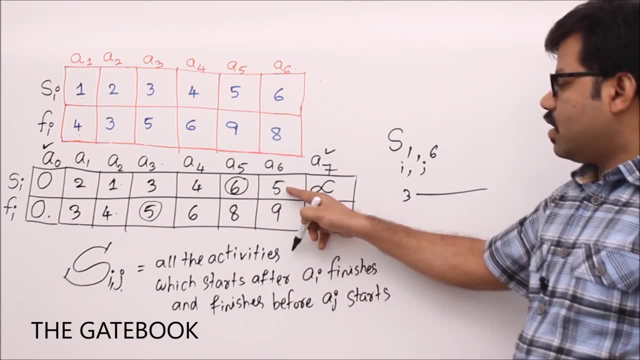 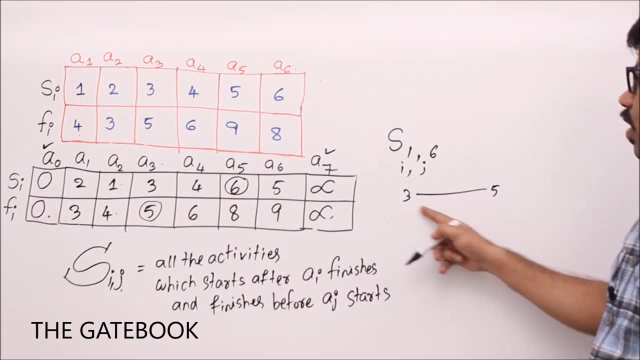 before a6 starts. a6 starts when a6 starts. 5, 3 to 5. is there any activity in between 3 to 5? yes, a3, anything else, no, right you so only one. in that way, we can find out sij any sij. now let's come to the problem, since these are: 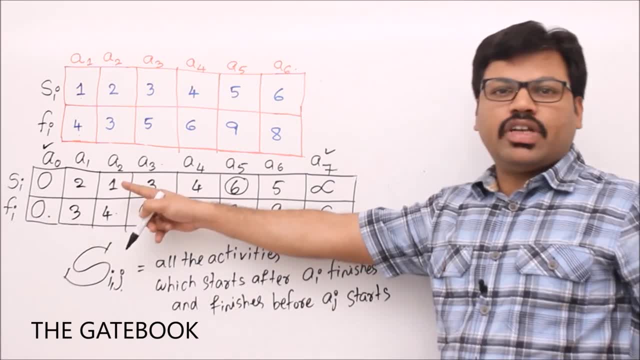 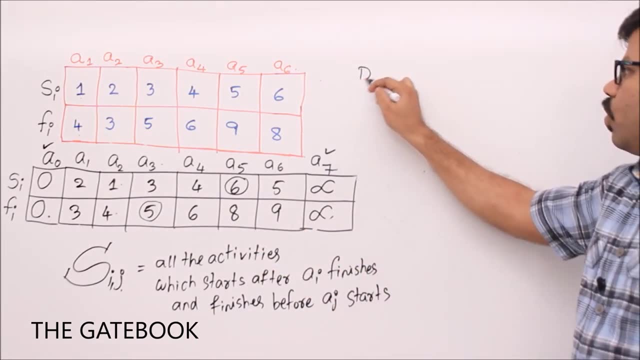 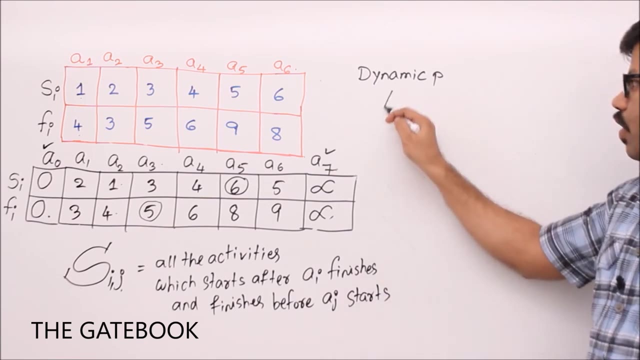 and one more thing you remember: we have sorted the elements or activities based on their finishing times. remember it. now we'll come to solution. i am going to give you dynamic programming solution with respect to this s. okay, so dynamic programming solution. what is that is? for that again, i use one another notation: a. a is our answer. what is this? s is just this.